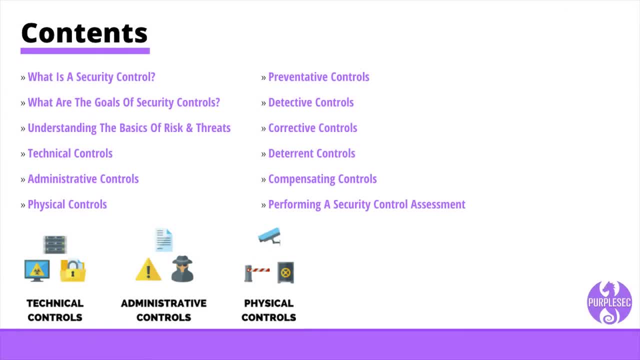 In this video, I'm going to explain what a security control is and the differences between each type. Next, I'll discuss the goals that each control is meant to achieve, with examples along the way. By the end, you'll have a better understanding of the basic security controls in cybersecurity. 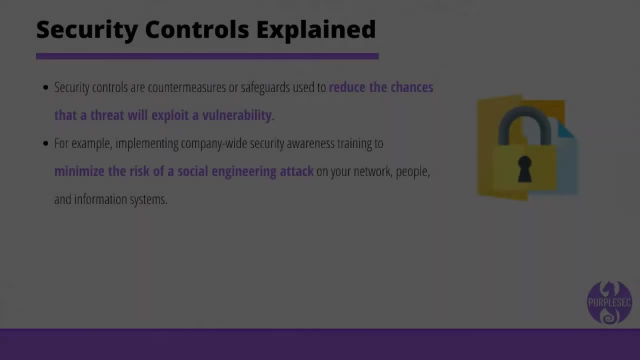 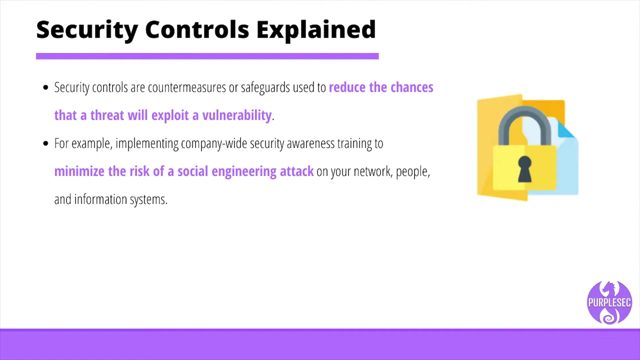 What is a security control? Security controls are countermeasures or safeguards used to reduce the chances that a threat will exploit a vulnerability, For example, implementing company-wide security awareness training to minimize the risk of a threat. The goal is to reduce the risk of a social engineering attack on your network, people and information systems. 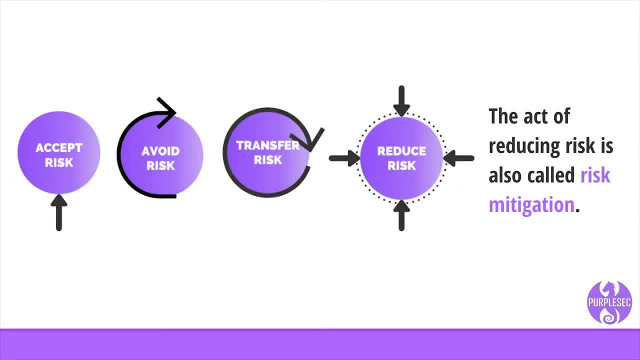 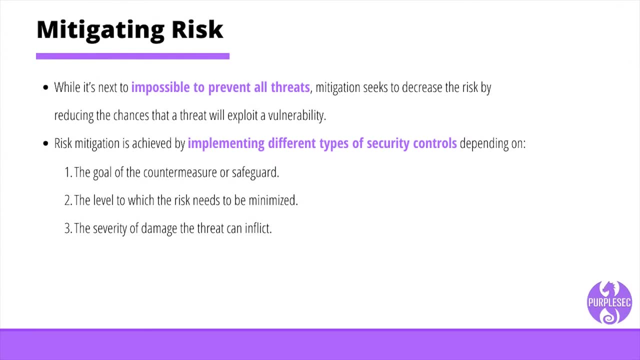 The act of reducing risk is also called risk mitigation. While it's next to impossible to prevent all threats, mitigation seeks to decrease the risk by reducing the chances that a threat will exploit a vulnerability. Risk mitigation is achieved by implementing different types of security controls. 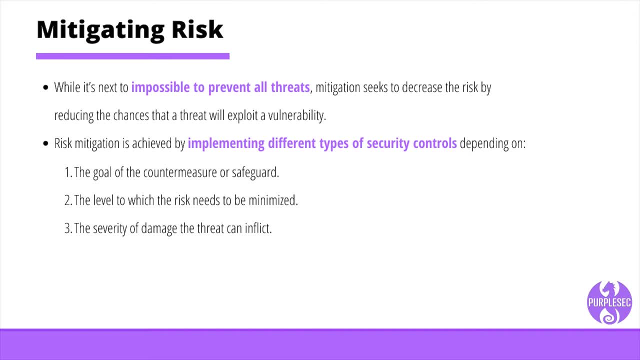 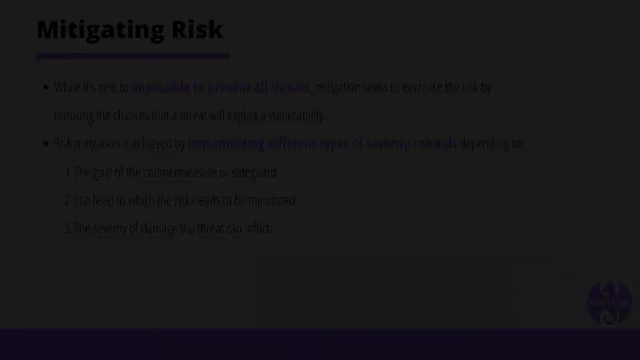 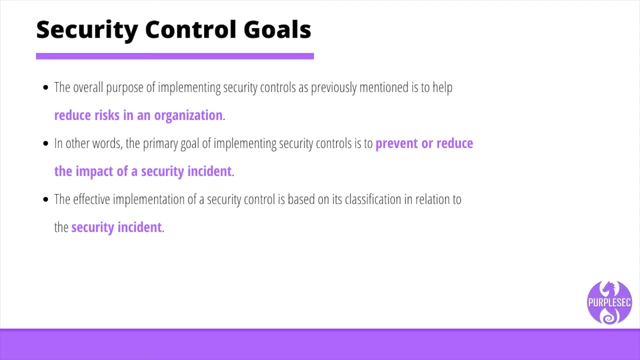 1. The goal of the countermeasures or safeguards. 2. The level to which the risk needs to be minimized. 3. The severity of damage the threat can inflict. What are the goals of security controls? The overall purpose of implementing security controls, as previously mentioned, is to help reduce risks in an organization. 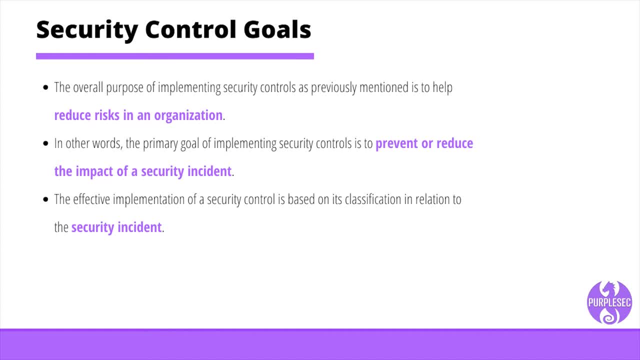 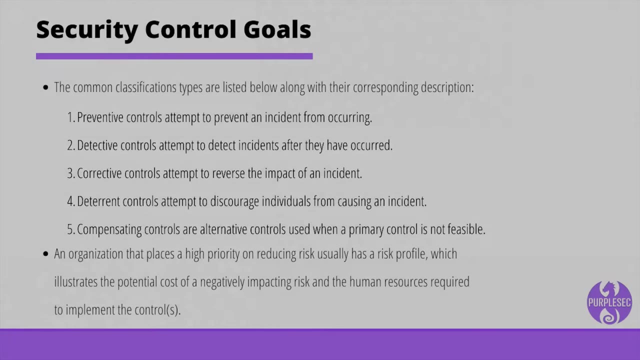 In other words, the primary goal of implementing security controls is to prevent or reduce the impact of a security incident. The effective implementation of a security control is based on its classification in relation to the security incident. The common classification types are listed below, along with their corresponding description. 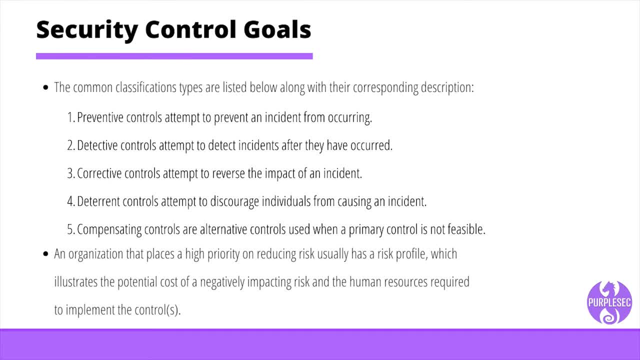 Preventative controls attempt to prevent an incident from occurring. Detective controls attempt to prevent an incident from occurring. Corrective controls attempt to detect incidents after they have occurred. Corrective controls attempt to reverse the impact of an incident. Deterrent controls attempt to discourage individuals from causing an incident. 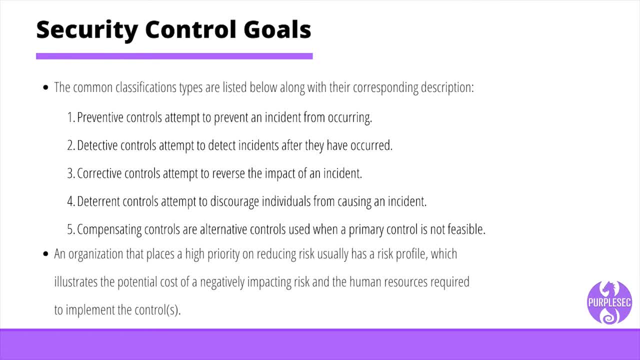 Compensating controls are alternative controls used when a primary control is not feasible. Implementing the controls listed is no trivial matter. For example, an organization that places a high priority on reducing risk usually has a risk-free system. The risk profile illustrates the potential cost of a negatively impacting risk and the human resources required to implement the controls. 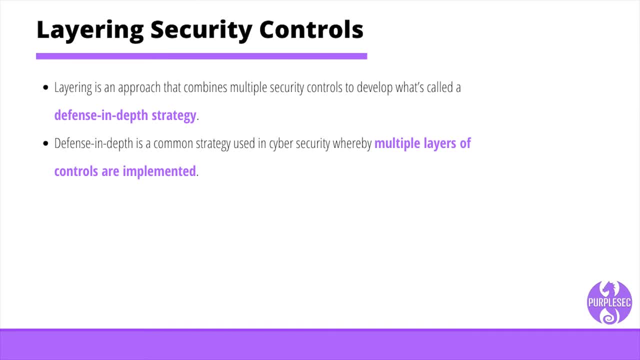 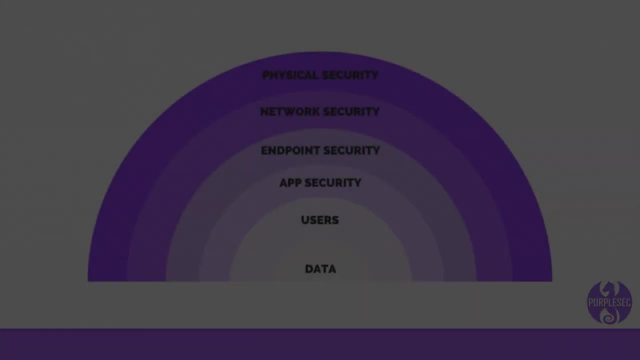 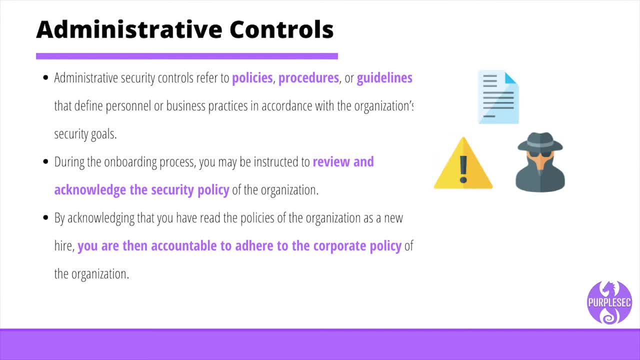 On the current onboarding process, you may be instructed to review and acknowledge the security policy of the organization. The status of the same organization is ilk By acknowledging that you have read the policies of the organization. as a new hire, you are then accountable to adhere to the corporate policy of the organization. 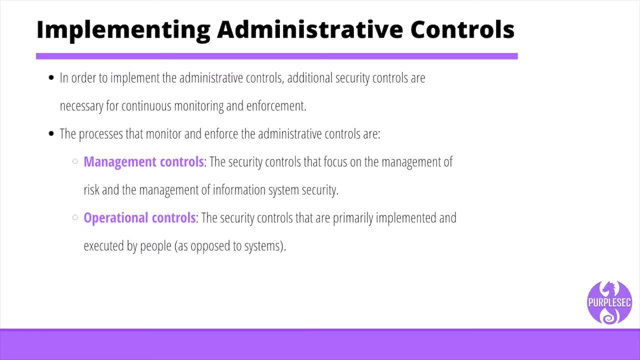 In order to implement the administrative controls, additional security controls are necessary for continuous monitoring and enforcement. 1- Management Controls: The processes and processes that monitor and enforce the administrative controls are Management Controls, which are security controls that focus on the management of information system security. Operational controls are security controls that are primarily implemented and executed by people. 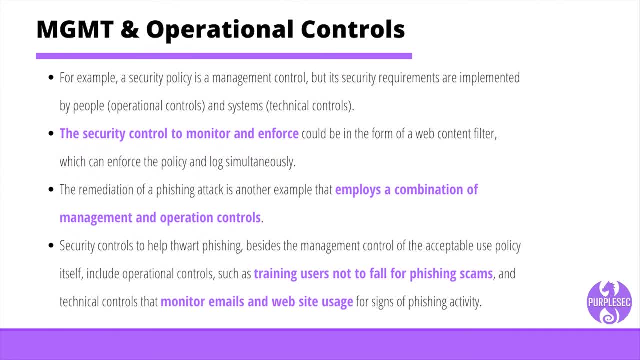 as opposed to systems. For example, a security policy is a management control, but its security requirements are implemented by people or operational controls and systems or technical controls. An organization may have an acceptable use policy that specifies the conduct of users. 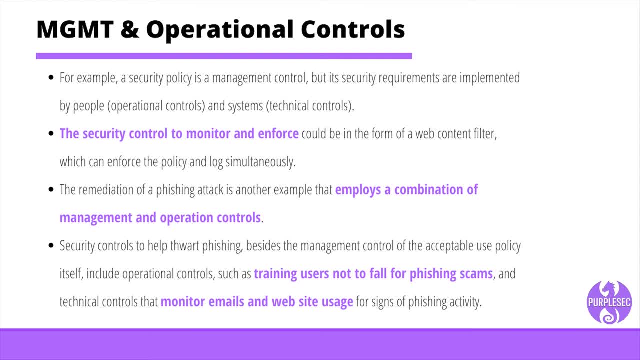 including not visiting malicious websites. The security control to monitor and enforce could be in the form of a web content filter which can enforce the policy and log simultaneously. The remediation of a phishing attack is another example that employs a combination of management and operation controls: Security controls to help thwart 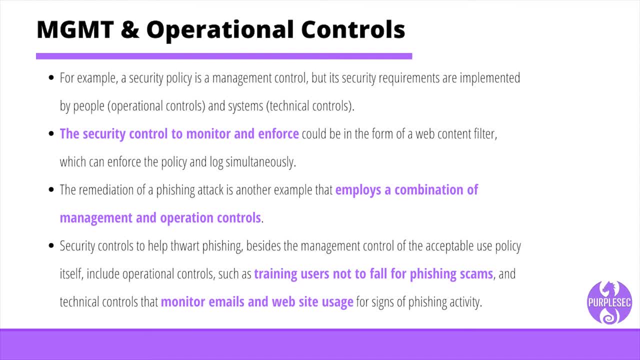 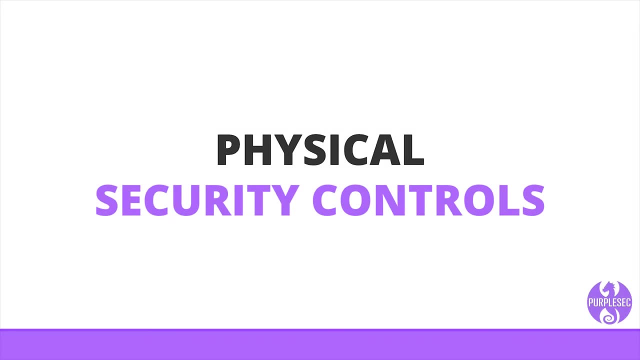 phishing are a combination of management and operational controls. Security controls to help thwart phishing, besides the management control of the acceptable use policy itself, include operational controls, such as training users not to fall for phishing scams, and technical controls that monitor emails and website usage for signs of phishing activity. Physical Security Controls: 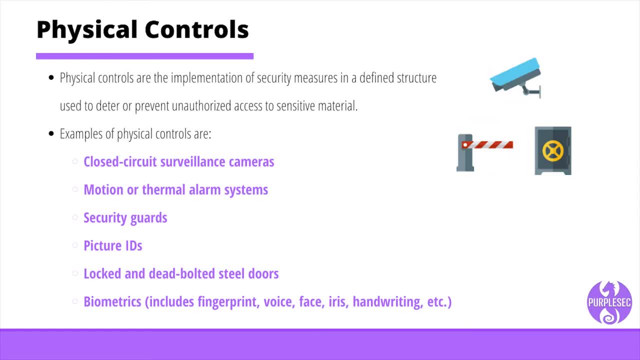 Physical controls are the implementation of security measures in a defined structure used to deter or prevent unauthorized access to sensitive material. Examples of physical controls are closed-circuit surveillance cameras, motion or thermal alarm systems, security guards, picture IDs, locked and deadbolted steel doors. 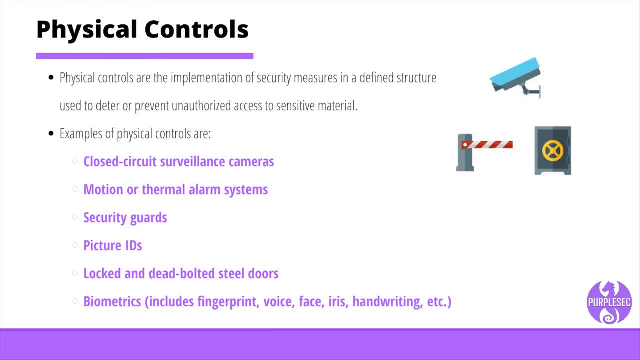 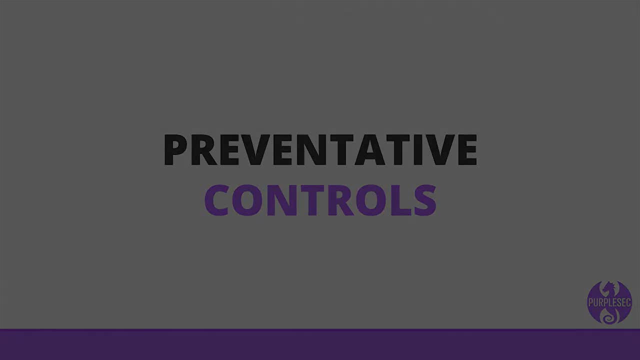 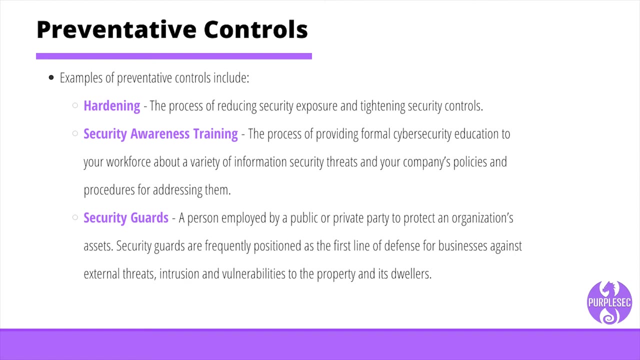 biometrics, including voice, face, iris or handwriting, and other automated methods used to recognize individuals. Preventative Controls. Examples of preventative controls include hardening security awareness, training security guards, change management and account disablement policy, Hardening The process of reducing security exposure and tightening security controls. 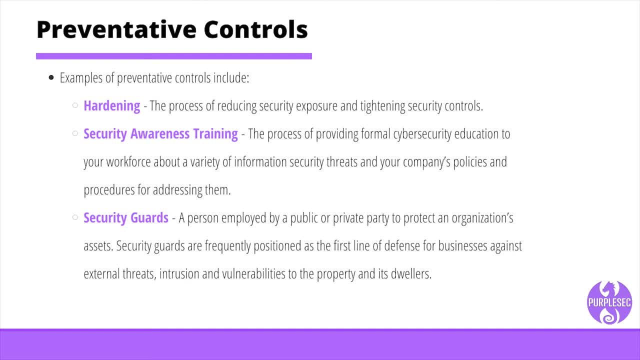 Security Awareness Training: The process of providing formal cybersecurity education to your workforce about a variety of information security threats and your company's policies and procedures for addressing them. Security Guards: A person employed by a public or private company to protect the organization's assets. Security guards are: 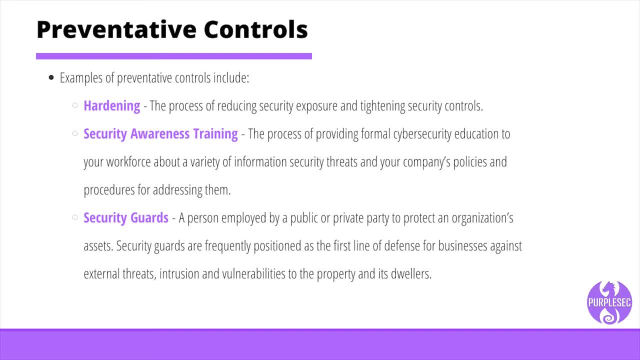 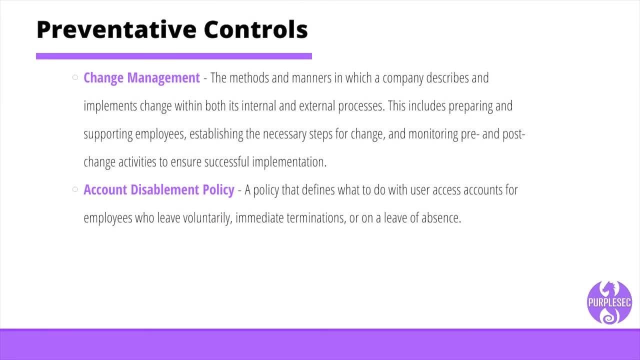 frequently positioned as the first line of defense for businesses against external threats, intrusions and vulnerabilities to the property and its dwellers. Change Management: The methods and manners in which a company describes and implements change within both its internal and external processes. This includes 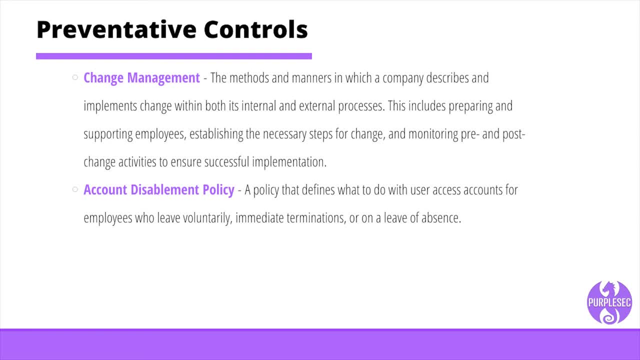 preparing and supporting employees, establishing the necessary steps for change and monitoring pre and post change activities to ensure successful implementation. Account Disablement Policy: A policy that defines what to do with users' access accounts for employees who leave voluntarily, immediately terminates or on a leave of absence. 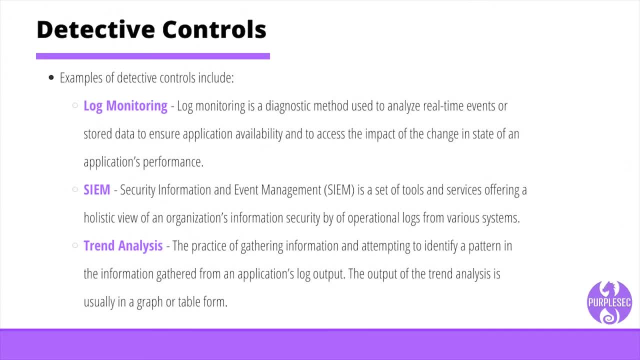 Detective Controls. Examples of detective controls include log monitoring, SIM trend analysis, security audits, video surveillance and motion detection. Log Monitoring: Log monitoring- is a diagnostic method used to analyze real-time events or stored data, to ensure application availability and to assess the impact of the change in state. 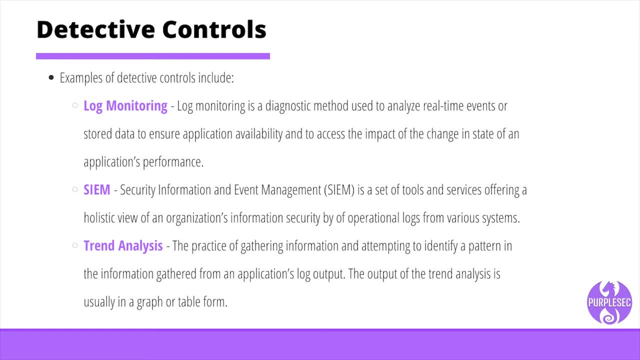 of an application's performance. SIEM, A security information and event management solution, supports threat detection, compliance and security incident management through the collection and analysis of security events, as well as a wide variety of other event and contextual data sources, Trend Analysis, The practice of gathering information and attempting to identify a pattern. 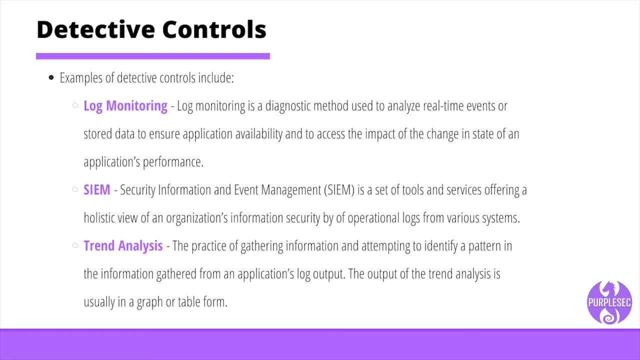 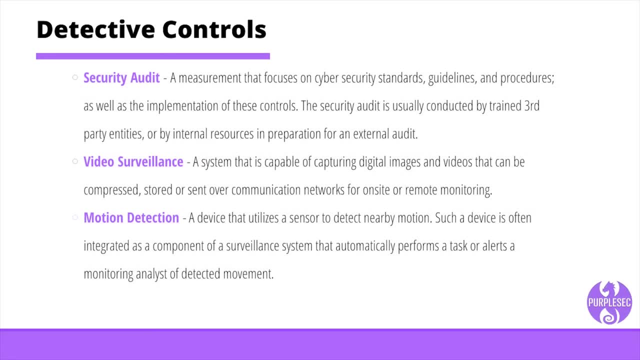 in the information gathered from an application's log output. The output of the trend analysis is usually in a graphic or table form. Security Audit: A measurement that focuses on security security standards, guidelines and procedures, as well as the implementation of these controls. 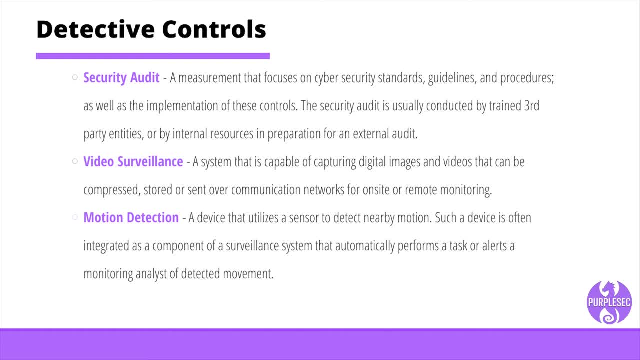 The security audit is usually conducted by trained third-party entities or by internal resources in preparation for an external audit. Video Surveillance: A system that is capable of capturing digital images and videos that can be compressed, stored or sent over communication networks for on-site or remote monitoring. 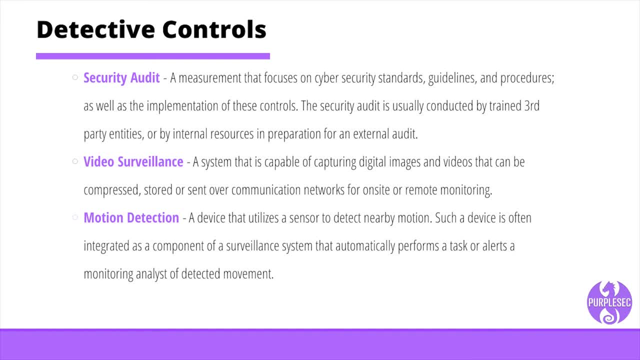 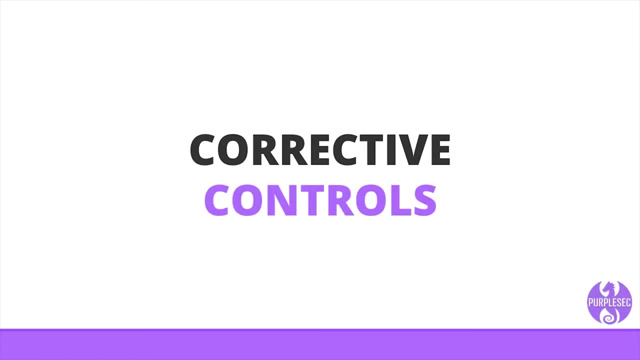 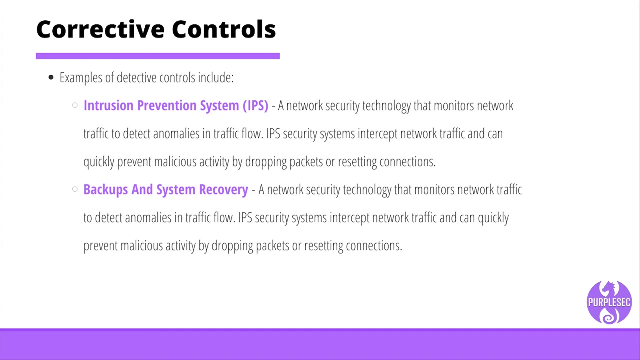 Motion Detection: A device that utilizes a sensor to detect nearby motion, such as a device, is often integrated as a component for a surveillance system that automatically performs a task or alerts a monitoring analyst of detected movement Corrective Controls. Examples of corrective controls include IPS, backups and recovery systems. 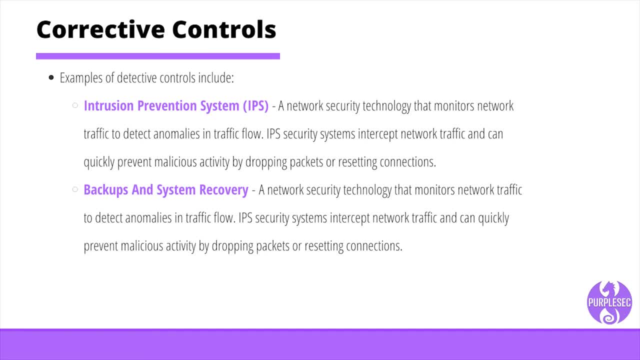 IPS, An intrusion prevention system, is a network security technology that monitors network traffic to detect anomalies in traffic flow. IPS security systems intercept network traffic and can quickly prevent malicious activity by dropping packets or resetting connections. Backups and System Recovery. Backups and system recovery is: 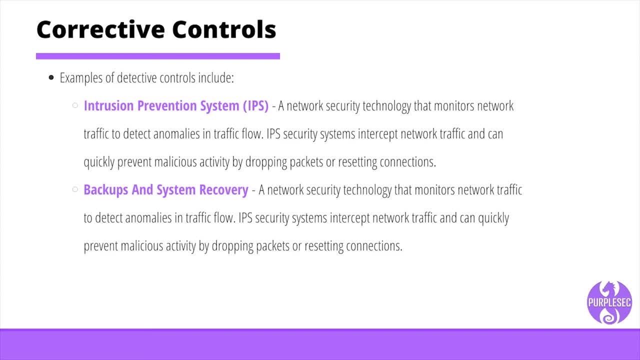 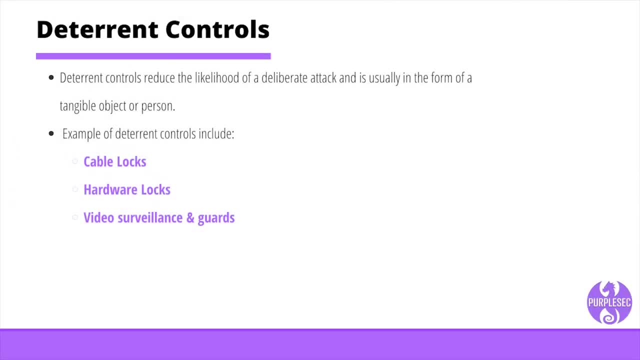 the process of creating and storing copies of data that can be used to protect organizations against data loss. Deterrent Controls- Deterrent Controls. Deterrent controls reduce the likelihood of a deliberate attack and is usually in the form of a tangible object or person. 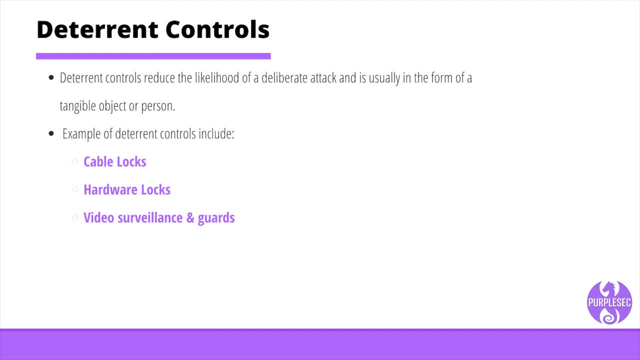 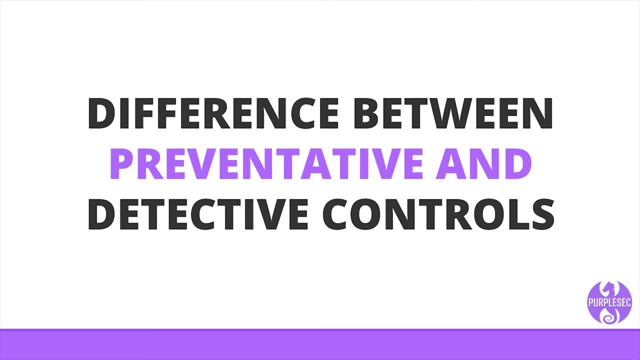 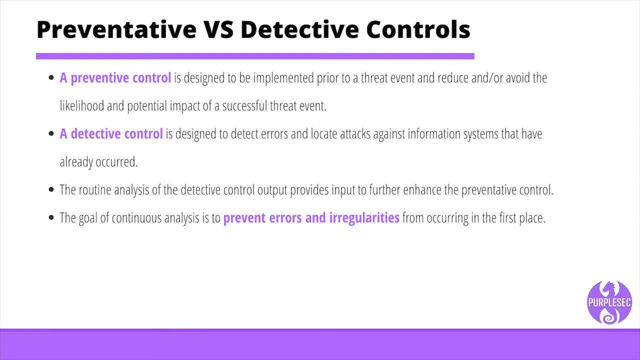 Deterrent Controls: radio Median Reductions. Deterrent controls is designed to be integrated, prioritized and pragmatized in dark and friendly approach In response to a controlled intervention. Detective control is designed to detect errors and locate attacks against information systems. 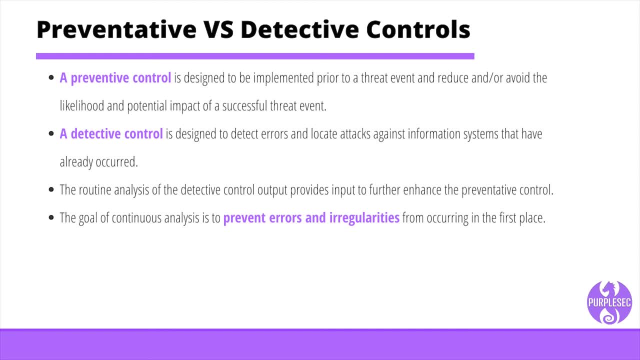 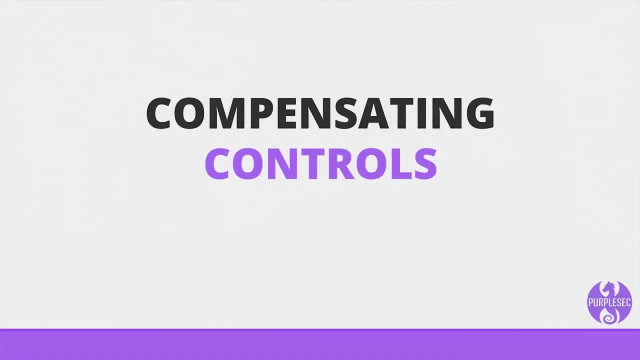 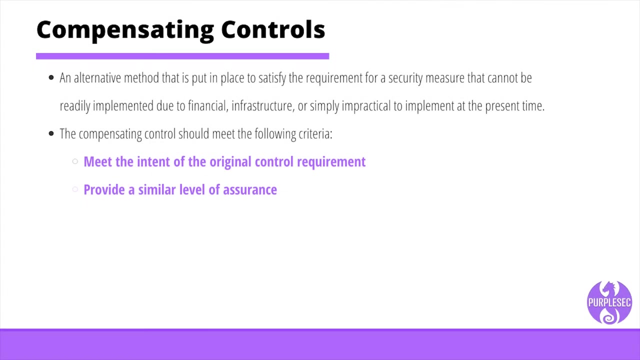 that have already occurred. The routine analysis of the detective control output provides input to further enhance the preventative control. The goal of continuous analysis is to prevent errors and irregularities from occurring in the first place. Compensating Controls An alternative method that is put in place to satisfy the requirement for a security 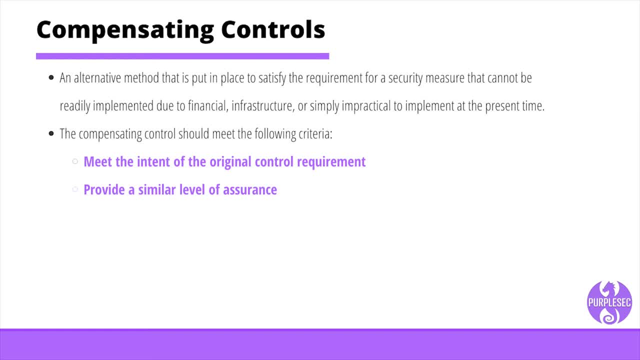 measure that cannot be readily implemented due to financial infrastructure or simply impractical to implement at the present time. The compensating control should meet the following criteria: Meet the intent of the original control requirement or provide a similar level of assurance. Examples of compensating controls include: 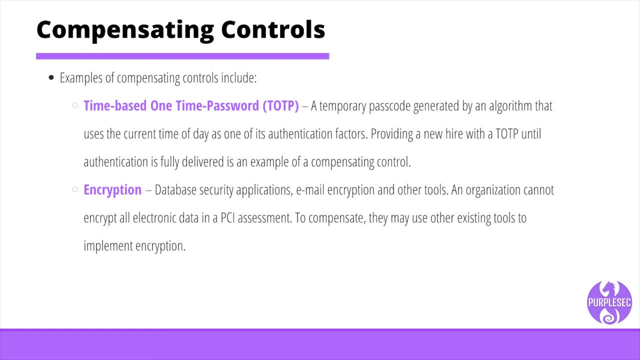 Time-based one-time passwords, or TOs, A temporary passcode generated by an algorithm that uses the current time of day as one of its authentication factors. Providing a new hire with a TOTP until authentication is fully delivered is an example of a compensating control. 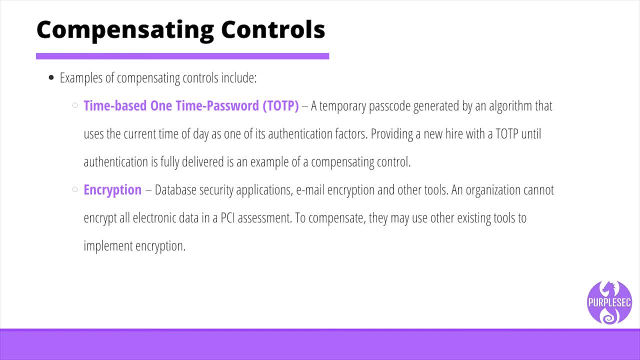 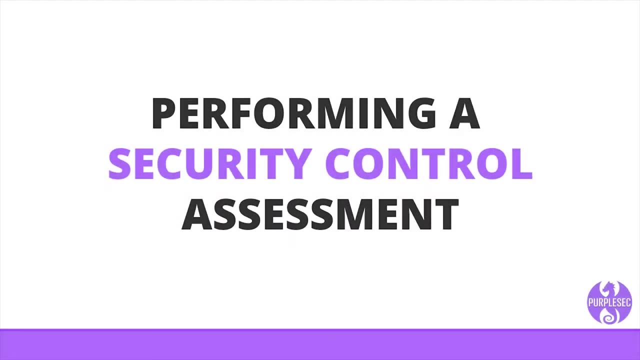 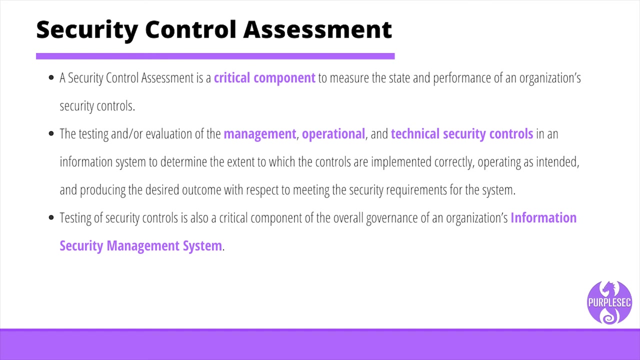 Encryption, Data-based security applications, email encryption and other tools. An organization cannot encrypt all electronic data in a PCI assessment. To compensate, they may use other existing tools to implement encryption. Performing a Security Control Assessment: A security control assessment is a critical component to measure the state and performance. 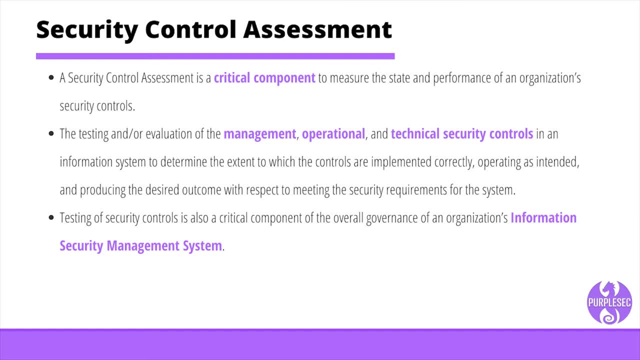 of an organization's security controls. Note the following definition of the security control assessment: The testing and or evaluation of the management, operational and technical security controls in an information system to determine the extent to which the security controls are used. The testing, evaluation and technical security controls should determine the extent to which 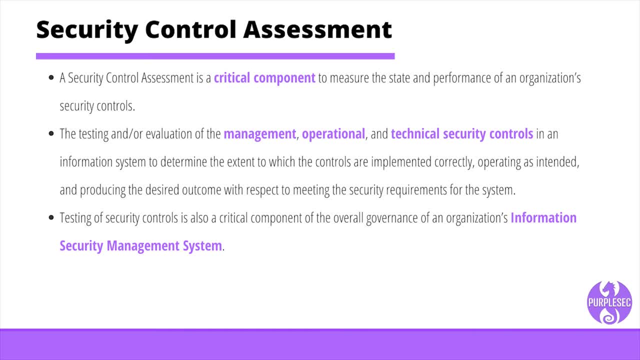 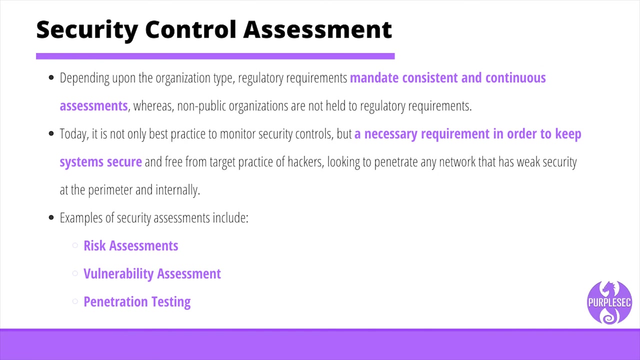 the controls are implemented correctly, operating as intended and producing the desired outcome with respect to meeting the security requirements for the system. Testing of security controls is a critical component of the overall governance of an organization's information security management system. Depending upon the organization type, regulatory requirements mandate consistent and continuous. 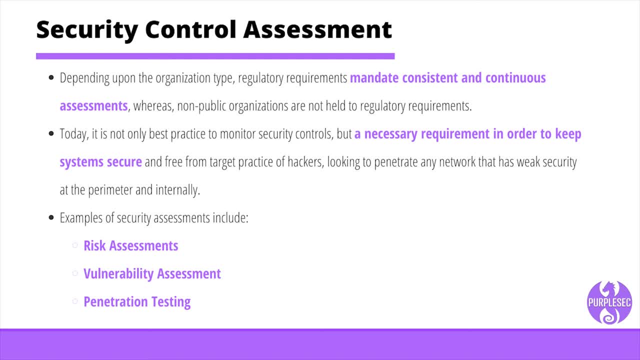 assessments, whereas non-public organizations are not held to regulars. So regulators must ensure that their service is not damaged or influenced by transactions and their legal processes. regulatory requirements: Today, it is not only best practice to monitor security controls, but a necessary requirement. 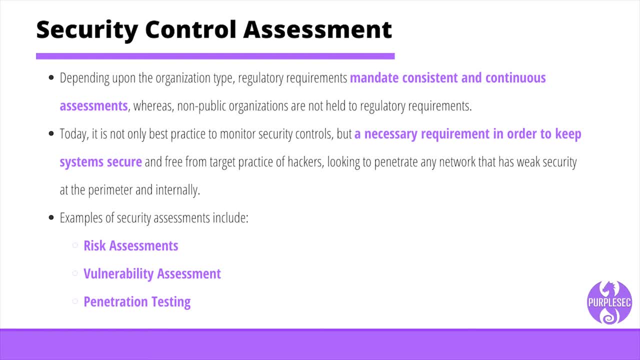 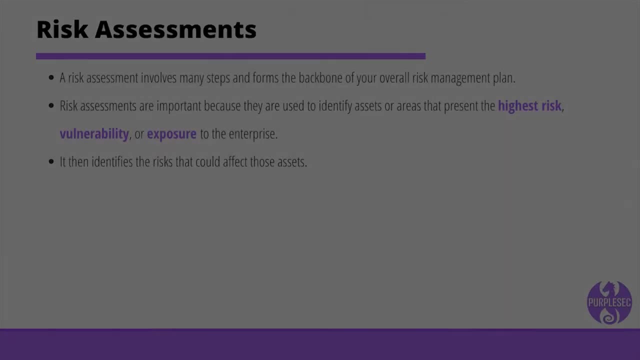 in order to keep systems secure and free from target practice of hackers looking to penetrate any network that has weak security at the perimeter and internally. Examples of security assessments include risk assessment, vulnerability assessment and penetration testing. A risk assessment involves many steps and forms the backbone of your overall risk management. 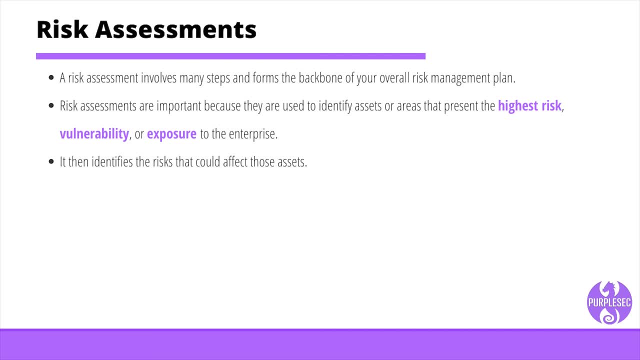 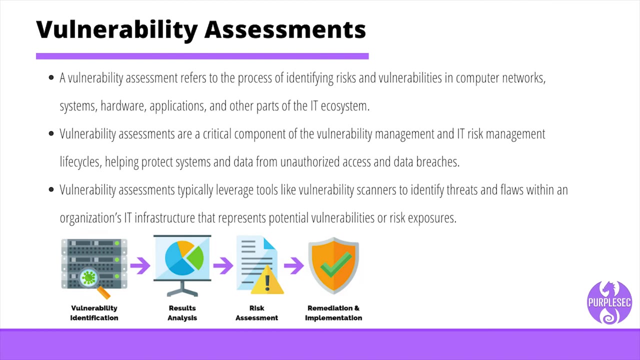 plan. Risk assessments are important because they are used to identify assets or areas that present the highest risk, vulnerability or exposure to the enterprise. It then identifies the risk that could affect those assets. Vulnerability assessments: A vulnerability assessment refers to the process of identifying risks and vulnerabilities. 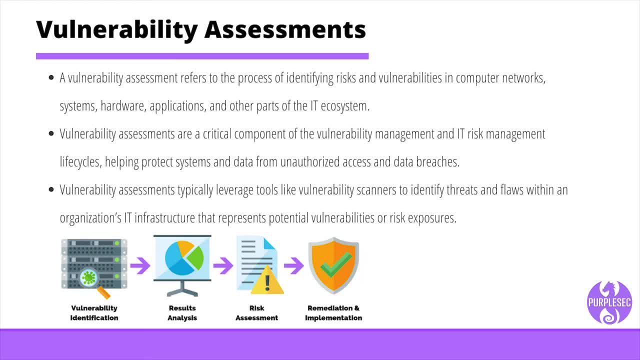 including computer networks, systems, hardware applications and other parts of the IT ecosystem. Vulnerability assessments are a critical component of the vulnerability management and IT risk management life cycles, helping protect systems and data from unauthorized access and data breaches. Vulnerability assessments typically leverage tools like vulnerability scanners to identify. 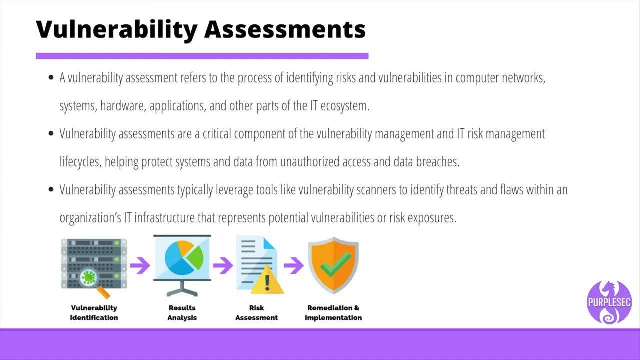 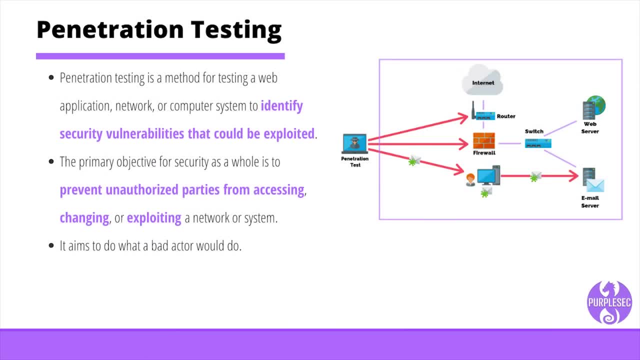 threats and flaws within an organization's IT infrastructure that represents potential vulnerabilities or risk exposure. Penetration testing is a method for testing a web application, network or computer system to identify security vulnerabilities that could be exploited. The primary objective for security as a whole is to prevent unauthorized parties from accessing, changing or exploiting a network or system. 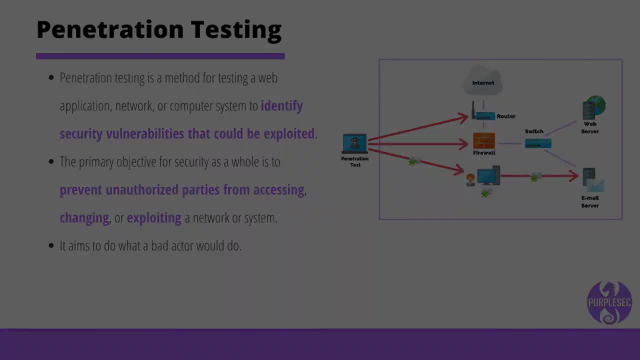 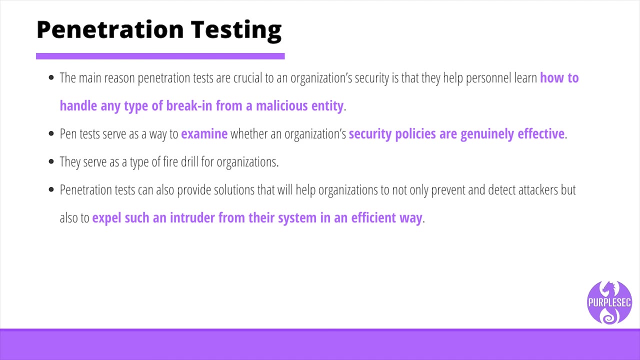 It aims to do what a bad actor would do. The primary reason penetration tests are crucial to an organization's security is that they help personnel learn how to handle any type of break-in from a malicious entity. Pen tests serve as a way to examine whether an organization's security policies are genuinely effective. 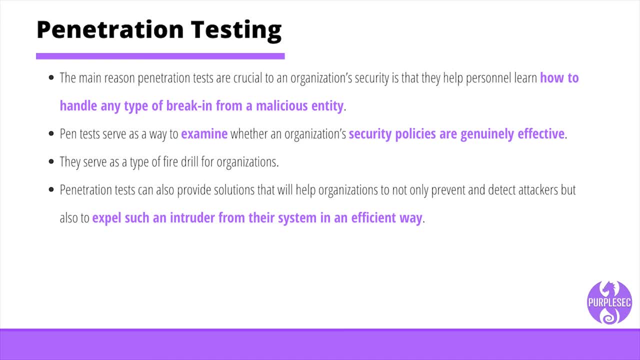 They serve as a type of fire drill for organizations. Penetration tests can also provide solutions that will help organizations to not only prevent and detect attackers, but also to expel unauthorized parties. A penetration test can also help organizations to not only prevent and detect attackers. 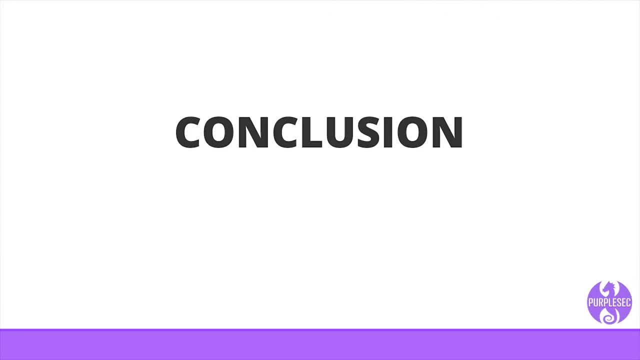 but also to expel unauthorized parties. Penetration tests can also provide solutions that will help organizations to not only prevent and detect attackers, but also to expel unauthorized parties. They serve as a way to examine whether an organization's security policies are genuinely effective.